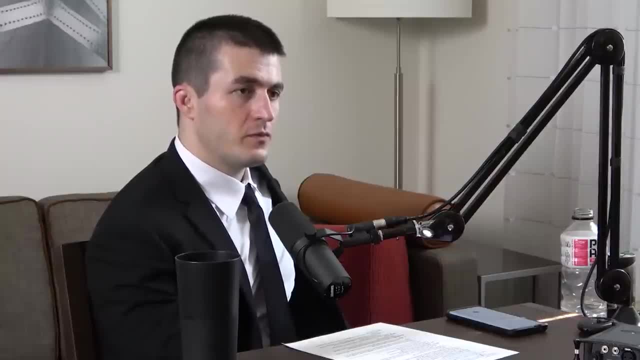 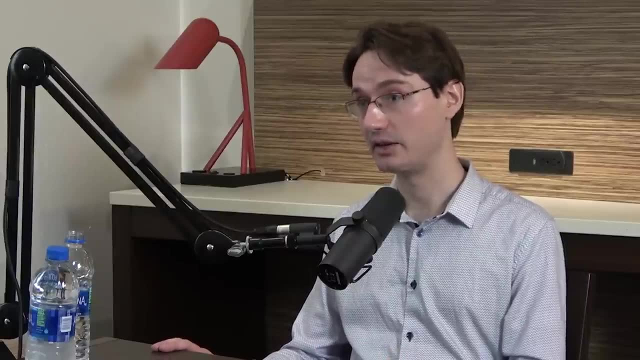 You must rotate the shape by 90 degrees. If I give you two examples and then I give you one prompt which is actually one of the two training examples, then there is zero generalization difficulty for the task. It's actually a trivial task. You just recognize that it's one of the 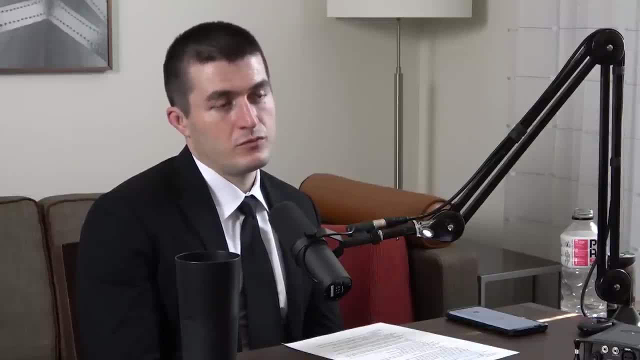 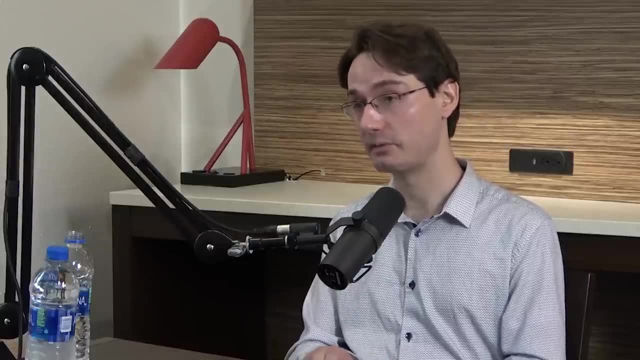 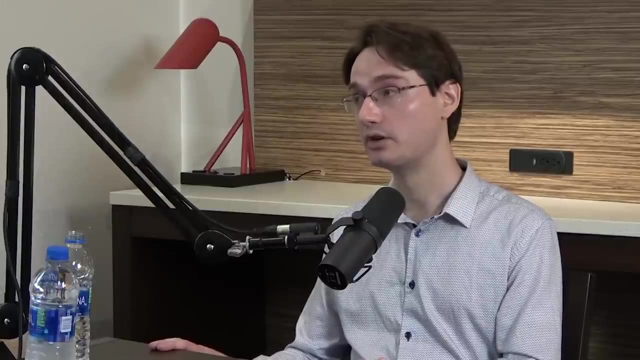 training examples and you produce the same answer. Now, if it's a more complex shape, there is a little bit more generalization, but it remains that you are still doing the same thing at this time as you were Being demonstrated at training time. a difficult task starts to require some amount of test time. 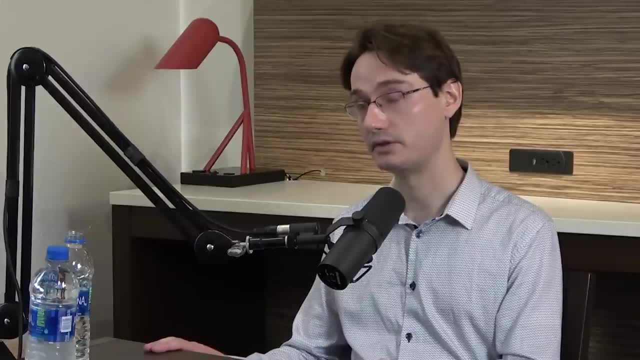 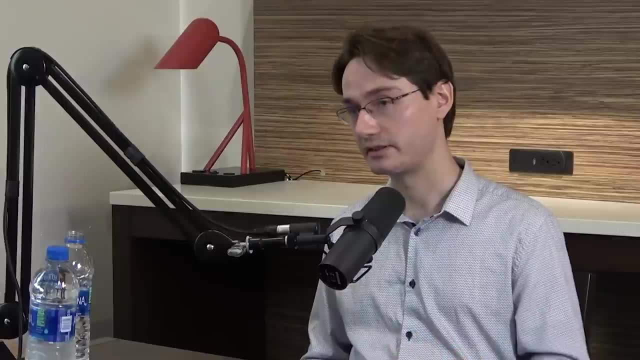 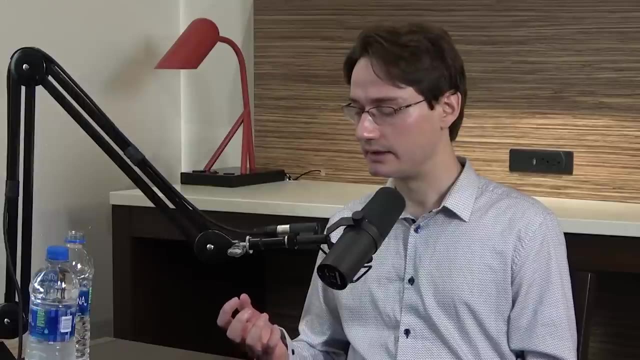 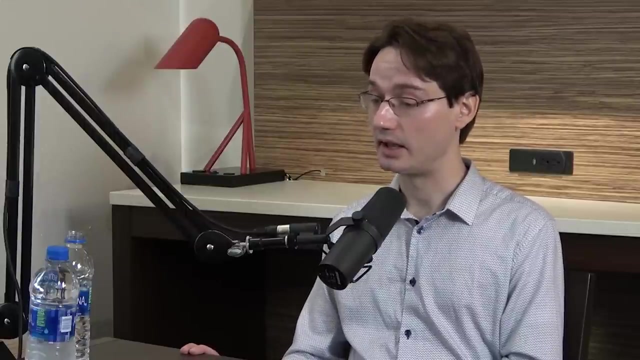 adaptation, some amount of improvisation, right? So consider: I don't know, you're teaching a class on quantum physics or something. If you wanted to test the understanding that students have of the material, you would come up with An exam that's very different from anything they've seen, like on the internet, when they 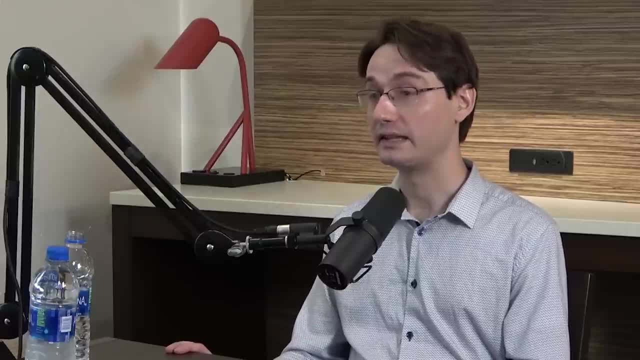 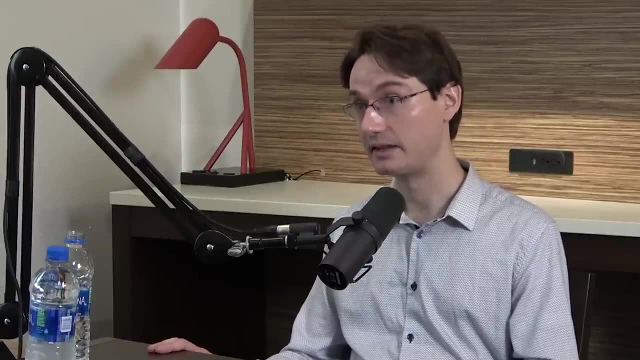 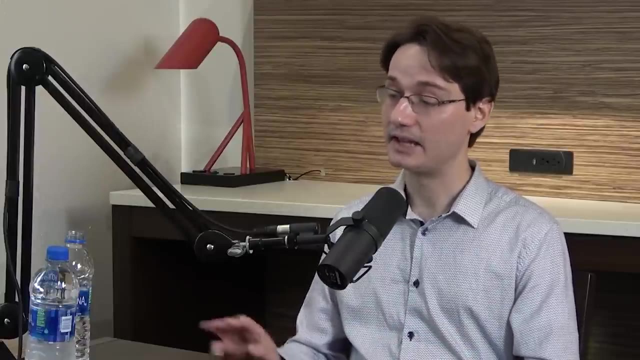 were cramming. On the other hand, if you wanted to make it easy, you would just give them something that's very similar to the mock exams that they've taken, something that's just a simple interpolation of questions that they've already seen, And so that would be an easy exam, It's. 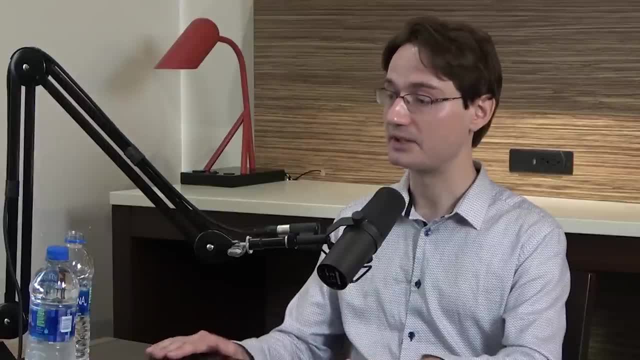 very similar to what you've been trained on, And a difficult exam is very similar to what you've been trained on, And a difficult exam is very similar to what you've been trained on, And a difficult exam is one that really probes your understanding, because it forces you. 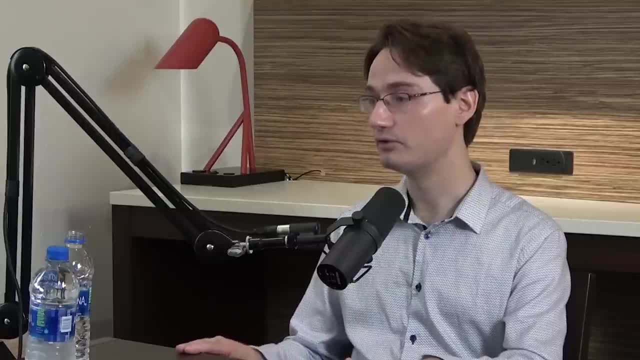 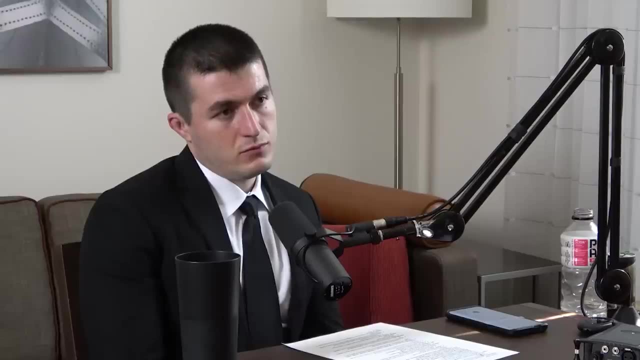 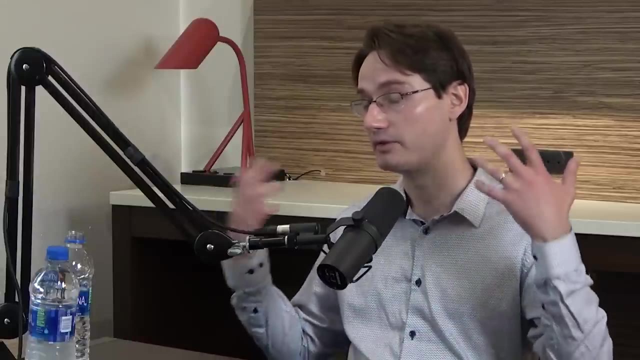 to improvise. It forces you to do things that are different from what you were exposed to before. So, that said, it doesn't mean that the exam that requires improvisation is intrinsically hard. right, Because maybe you're a quantum physics expert, So when you take the exam, 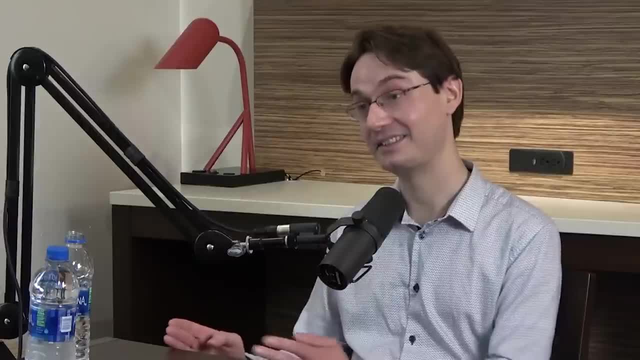 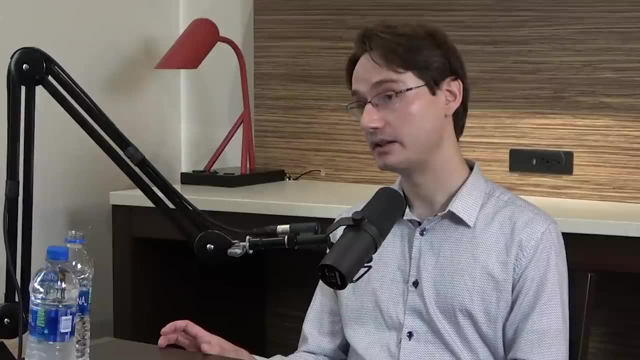 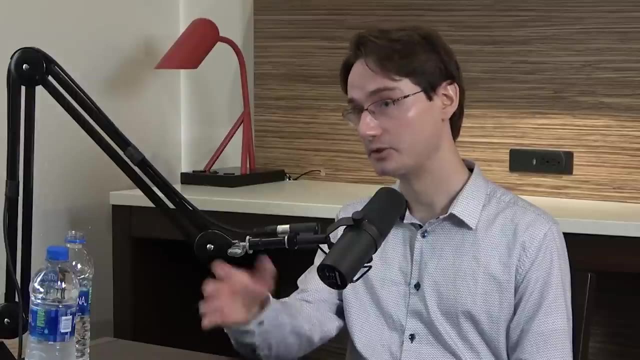 this is actually stuff that, despite being new to the students, it's not new to you, right? So it can only be difficult with respect to what the test taker already knows and with respect to the information that the test taker has about the task. So that's what I mean by controlling for. 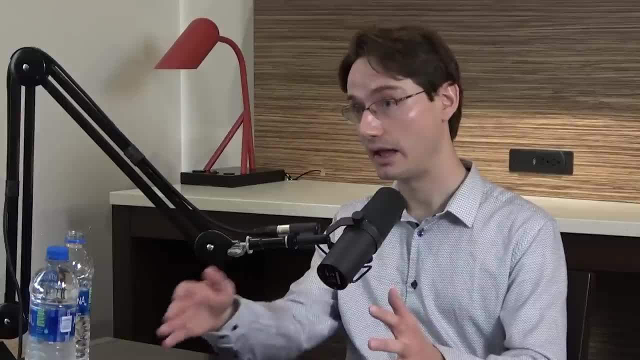 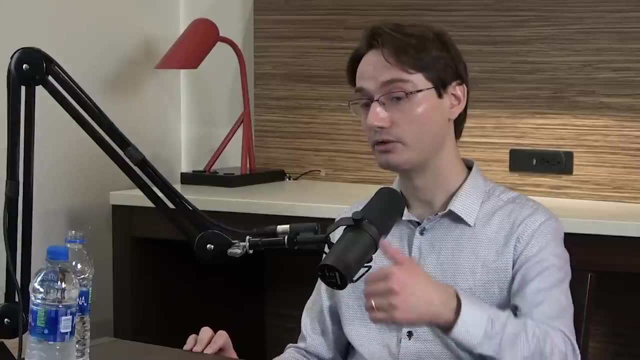 priors what you, the information you bring to the table and the experience, which is the training data. So, in the case of the quantum physics exam, that would be all the course material itself and all the mock exams that students might have taken online. 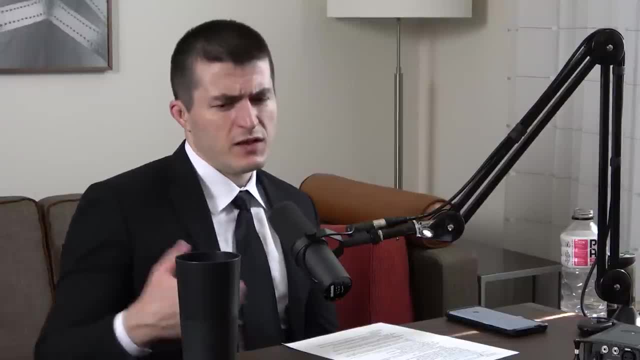 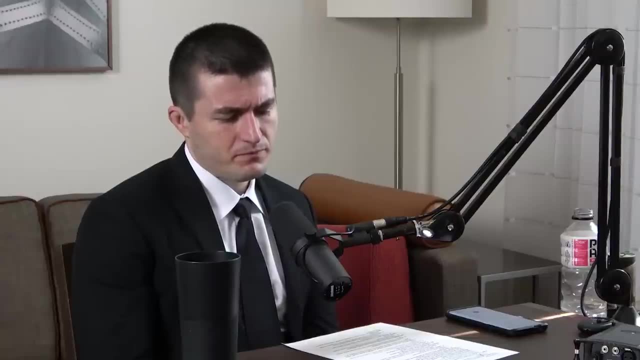 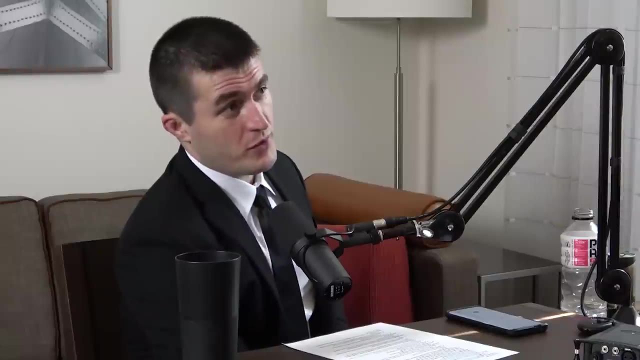 Yeah, it's interesting because I've also. I sent you an email and I asked you- like I've been just this curious question of you, know what's a really hard IQ test question? And I've been talking to also people who have designed IQ tests. There's a few folks on the internet. It's like a. 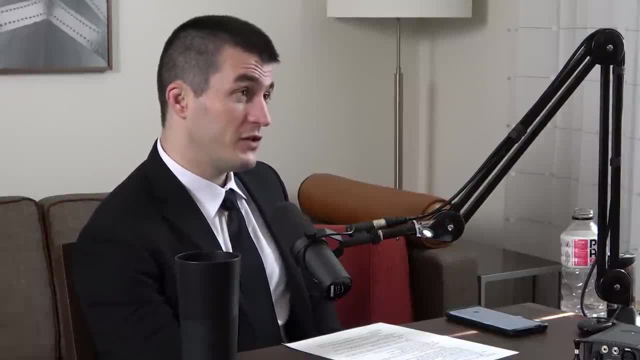 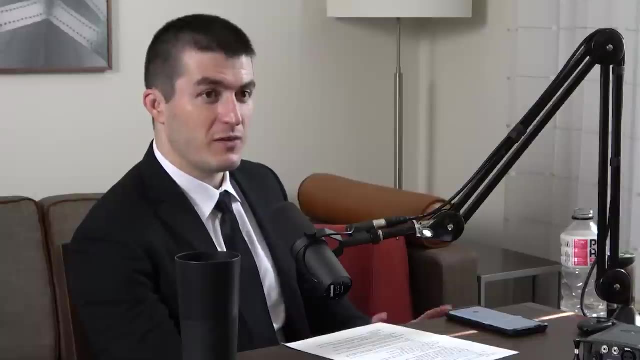 thing People are really curious about it. First of all, most of the IQ tests they designed, they like religiously, protect against the correct answers, Like you can't find the correct answers anywhere. In fact, the question is ruined once you know, even like, the approach you're supposed to take. 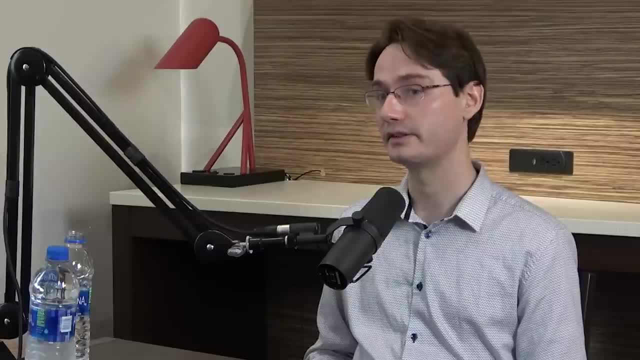 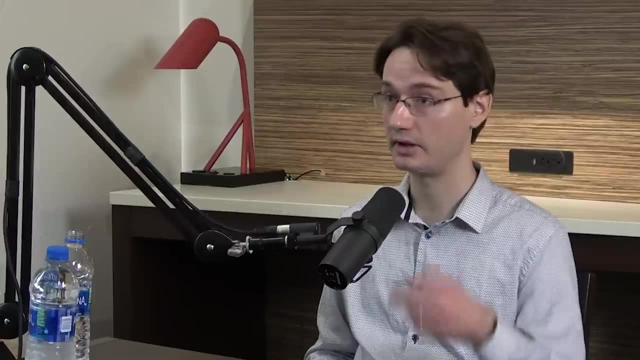 Mm-hmm. So they're very. That's the. the approach is implicit in in the training examples. So if you release the training examples, it's over. Well, Which is why in in Arc, for instance, there is a test set that is private and no one has seen it. 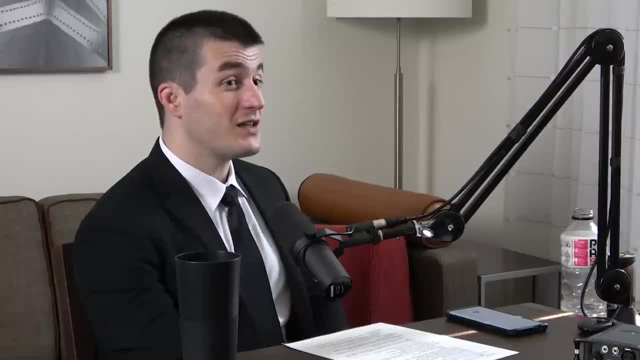 No For really tough IQ questions. it's not obvious. obvious it's not because the ambiguity like it's uh, i mean we have to look to them, but like some number sequences and so on. it's not completely clear so like you can get a sense, but there's. 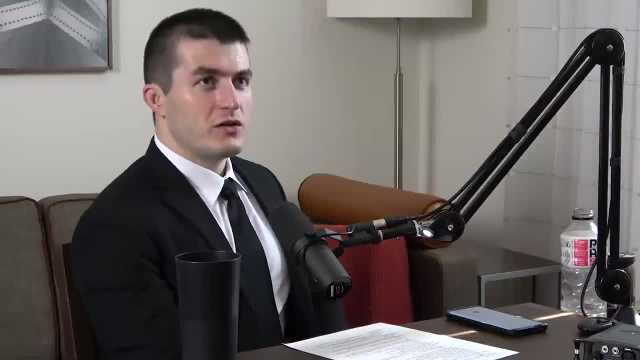 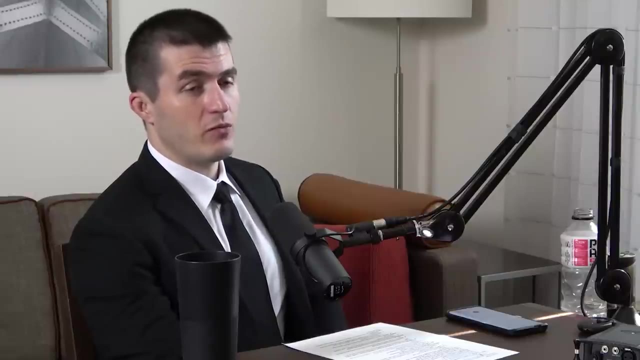 like some. you know, when you look at a number sequence- i don't know, uh, like your feminazi number sequence- if you look at the first few numbers, that sequence could be completed in a lot of different ways. and you know some are, if you think deeply, are more correct than others, like 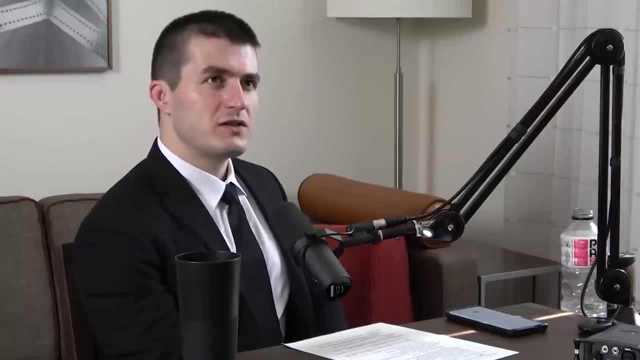 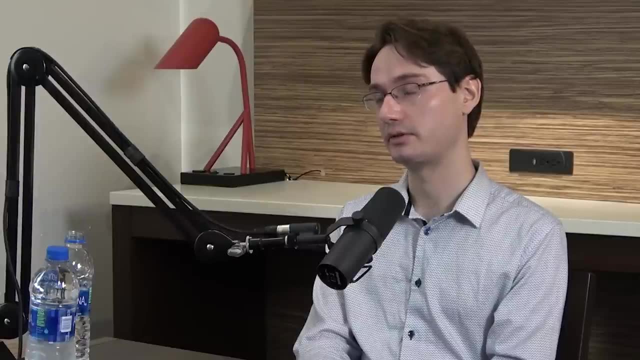 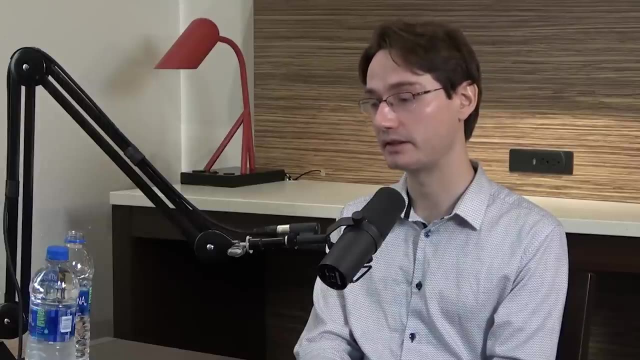 there's a kind of intuitive simplicity and elegance to the correct solution. yes, i am personally not a fan of ambiguity in in test questions actually- but i think you can have difficulty without requiring ambiguity simply by making the test require a lot of extrapolation over the training examples. but 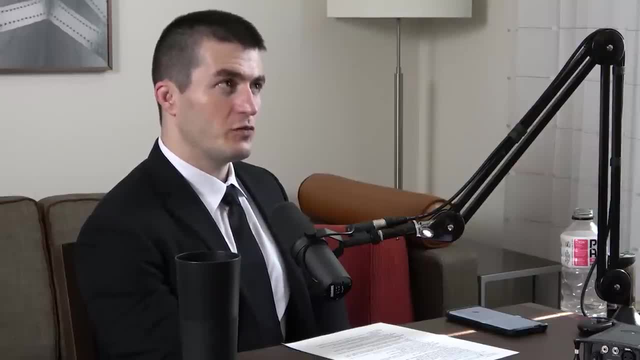 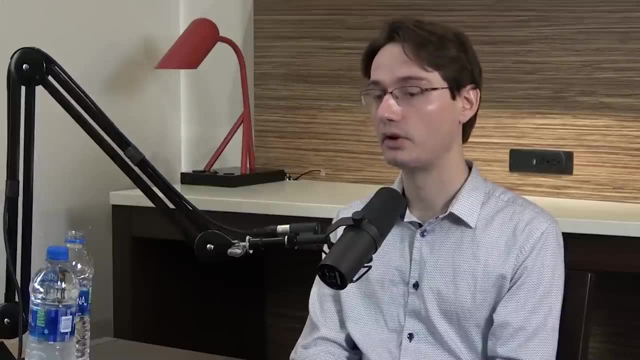 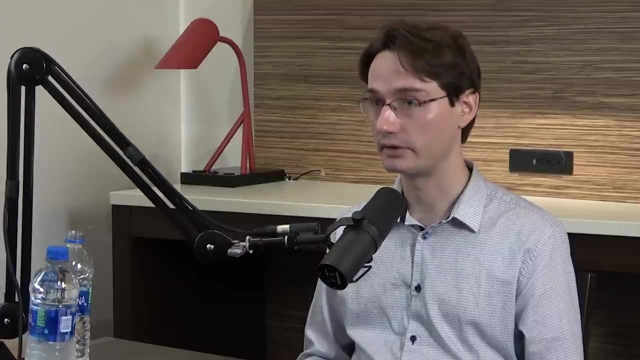 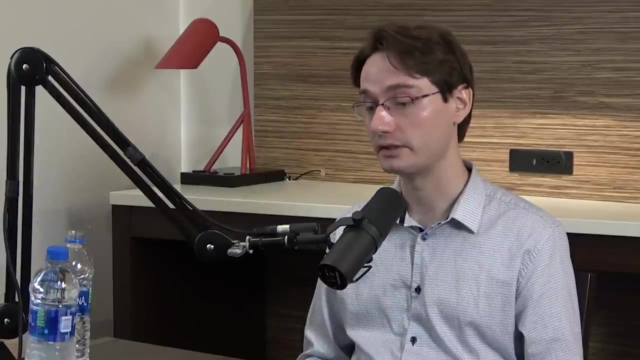 the, the beautiful question is difficult but gives away everything when you give the training example, basically yes, meaning that. so the, the, the tests i'm interested in in creating, are not necessarily difficult, uh for humans, because human intelligence is the benchmark. they're supposed to be difficult for machines in ways that are easy for humans, like, i think, an ideal uh test of human and machine. 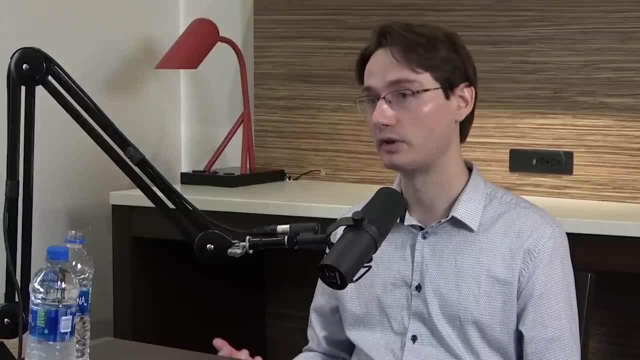 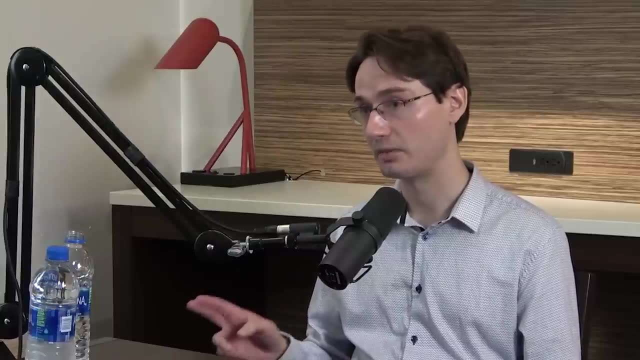 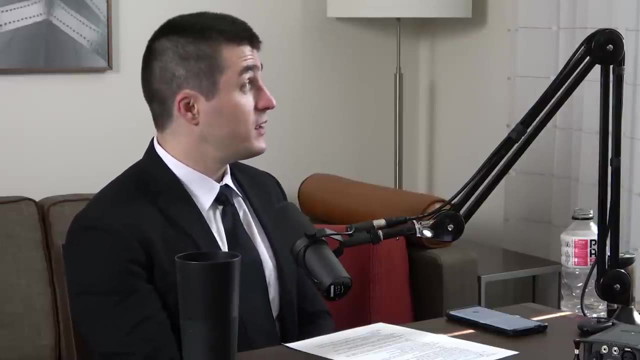 is a test that is, uh, actionable, uh, that highlights, uh, the need for progress and that highlights the direction in which you should be making progress. i- i think we'll talk about the arc challenge- and the test you've constructed is these elegant examples. i think that highlight, like this, is: 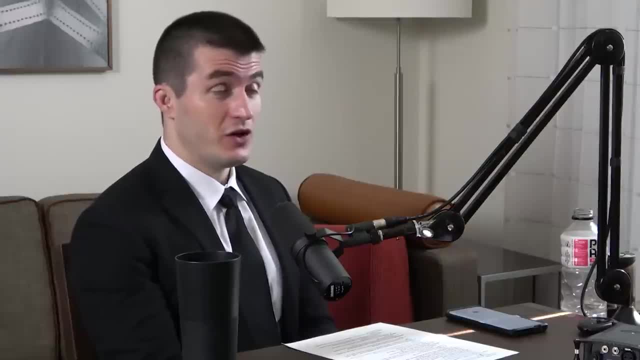 really easy for us humans but it's really hard for machines. but on the- you know the designing an iq test for iqs of like a higher than 160 and so on, you have to say you have to take that and put on steroids, right, you have to think like what is hard for humans. and that's a fascinating exercise in itself. 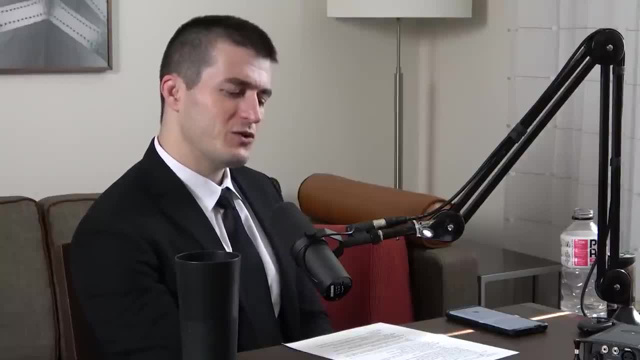 i think- and it was an interesting question- of what it takes to create a really hard question for humans because, um, you again have to do the same process, as you mentioned, which is, uh, you know, you have to do the same thing. um, basically, where the experience that you have likely to have? 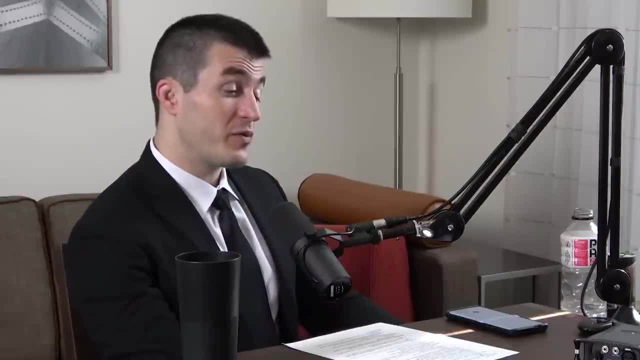 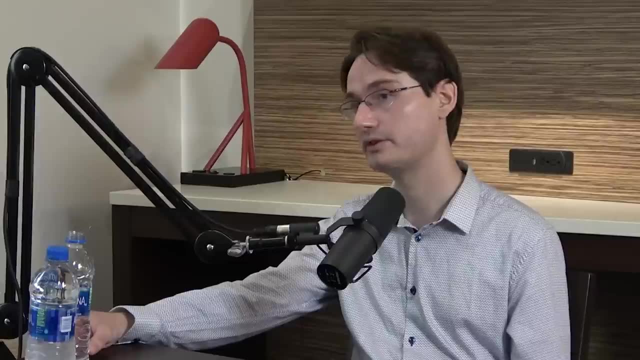 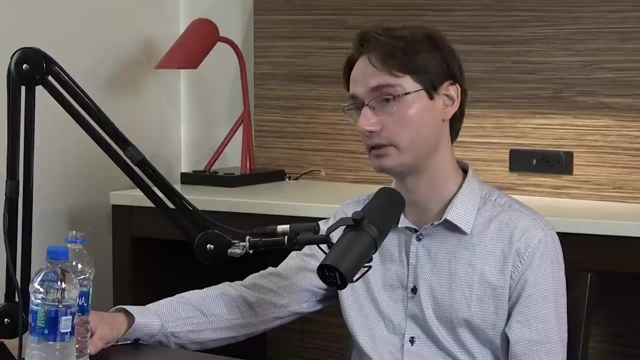 encountered throughout your whole life, even if you've prepared for iq tests, which is a big challenge- that this will still be novel for you. yeah, i mean, novelty is a requirement. uh, you should not be able to practice for the questions that you're going to be tested on, that's. 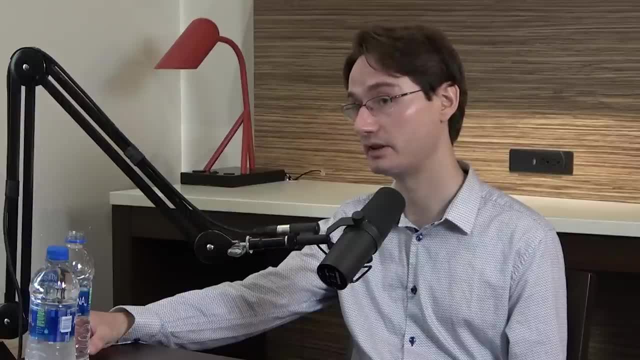 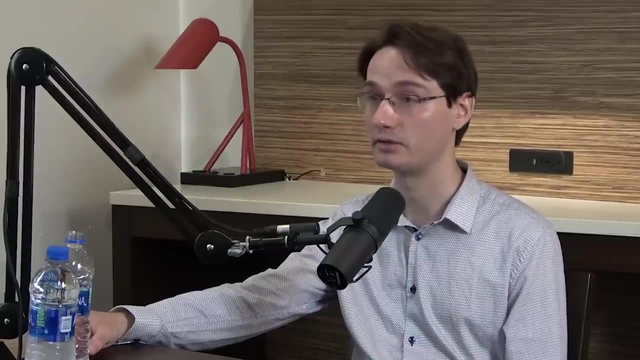 important, because otherwise what you're doing is not exhibiting intelligence. what you're doing is just retrieving the information that you're going to be testing on. that's important because otherwise what you're doing is not exhibiting intelligence. what you're doing is just retrieving- uh, what you've been exposed before. it's is the same thing as a deep learning model if you train.